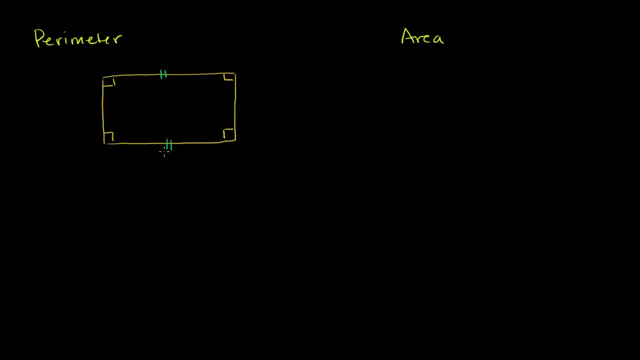 And the opposite sides are equal in length, So that side is going to be equal in length to that side and that side is equal in length to that side. And maybe I'll label the points A, B, C and D. 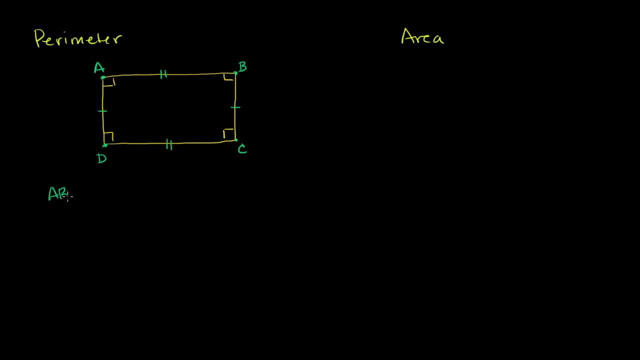 And let's say we know the following: We know that AB is equal to 7, and we know that BC is equal to 5.. And we want to know what is the perimeter of ABCD. So let me write down the perimeter of rectangle ABCD. 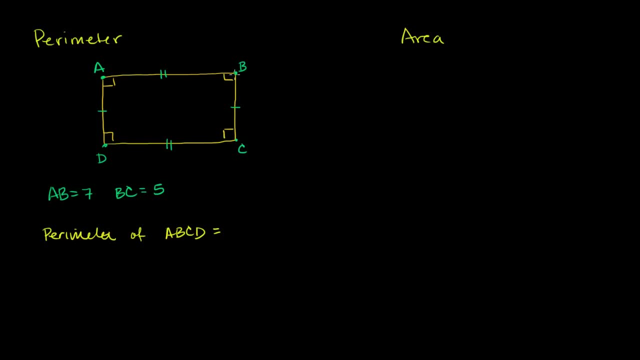 is just going to be equal to the sum of the lengths of the sides. If I were to build a fence, this was like a plot of land. I would just have to measure how long is this side right over here? Well, we already know. that's 7 in this color. 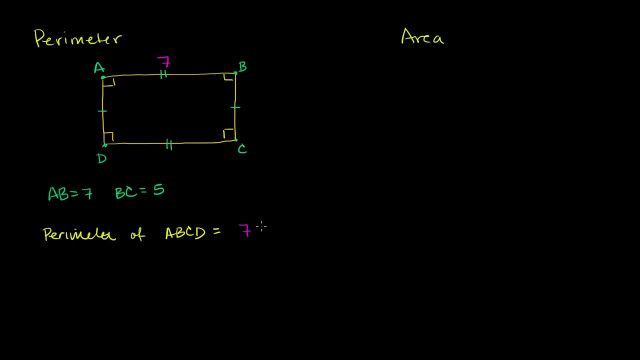 So that side right over there is of length 7.. So it'll be 7 plus this length over here which is going to be 5.. They tell us that BC is 5 plus 5 plus DC is going to be the same length as AB. 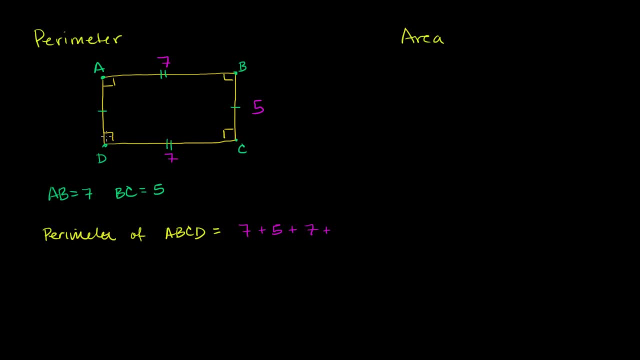 which is going to be 7 again, So plus 7.. And then finally, DA or AD, however you want to call it. OK, It's going to be the same length as BC, which is 5 again, So plus 5 again. 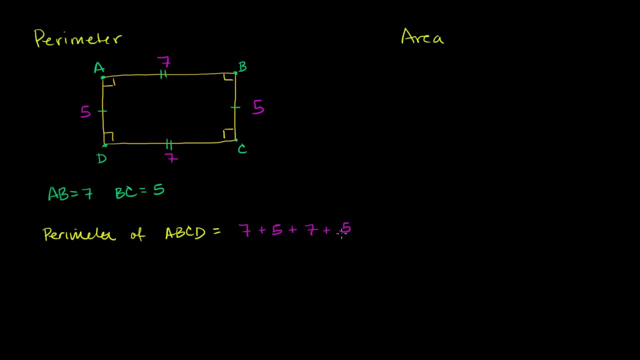 So you have: 7 plus 5 is 12 plus 7 plus 5 is 12 again, So you're going to have a perimeter of 24.. And you could go the other way around. Let's say that you have a square which. 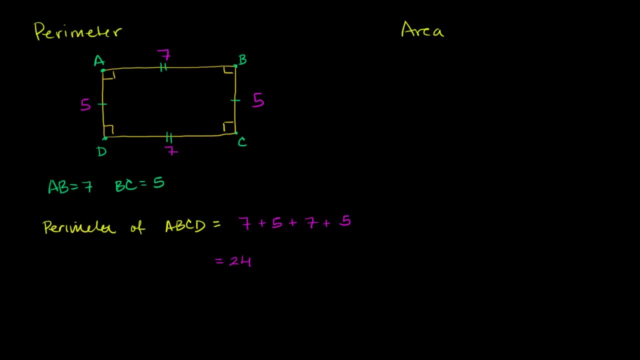 is a special case of a rectangle. A square has four sides and four right angles, and all of the sides are equal. So let me draw a square here, My best attempt. So this is ABCD And we're going to tell ourselves. 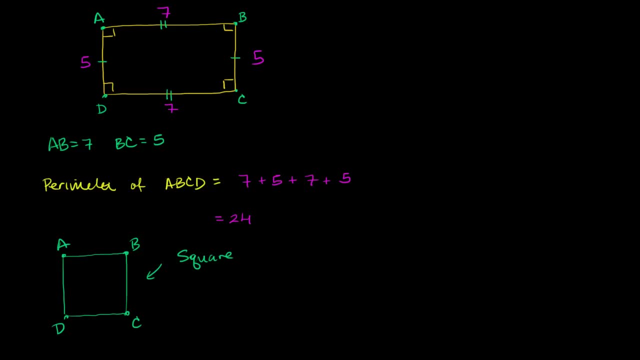 that this right here is a square And let's say that this square has a perimeter, So square has a perimeter of 36.. So, given that this square has a perimeter of 36, we're going to have 36.. OK, OK. 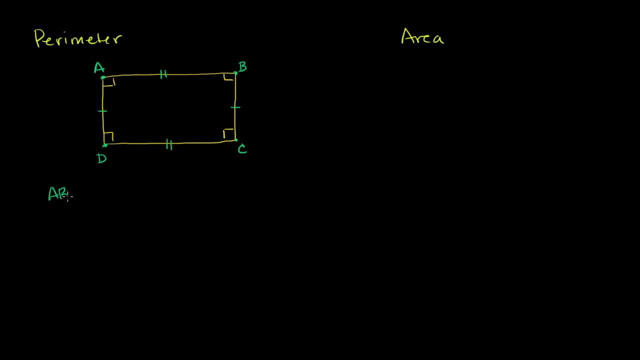 And let's say we know the following: We know that AB is equal to 7, and we know that BC is equal to 5.. And we want to know what is the perimeter of ABCD. So let me write down the perimeter of rectangle ABCD. 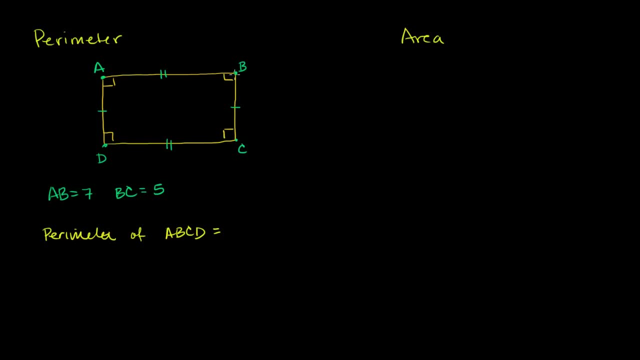 is just going to be equal to the sum of the lengths of the sides. If I were to build a fence, this was like a plot of land. I would just have to measure how long is this side right over here? Well, we already know. that's 7 in this color. 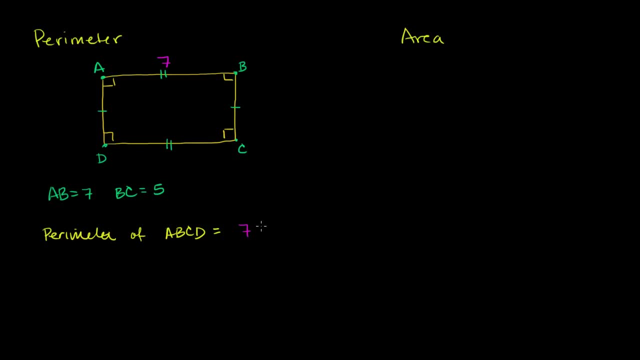 So that side right over there is of length 7.. So it'll be 7 plus this length over here which is going to be 5.. They tell us that BC is 5 plus 5.. Plus DC is going to be the same length as AB. 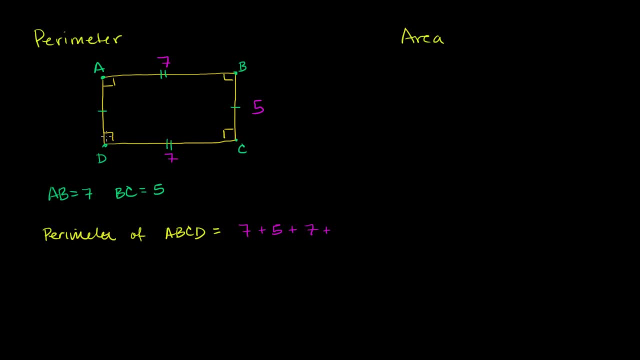 which is going to be 7 again, So plus 7.. And then finally, DA or AD, however you want to call it, It's going to be the same length as BC, which is 5 again, So plus 5 again. 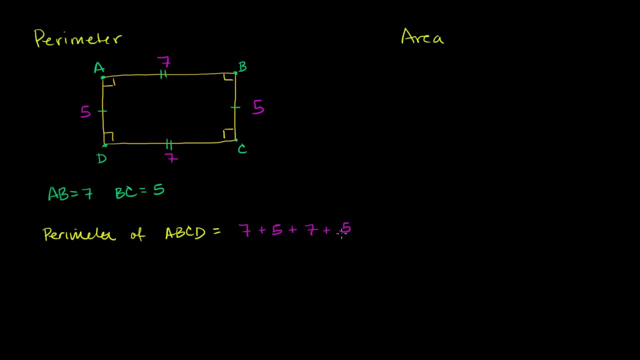 So you have: 7 plus 5 is 12, plus 7 plus 5 is 12 again, So you're going to have a perimeter of 24.. And you could go the other way around. Let's say that you have a square which. 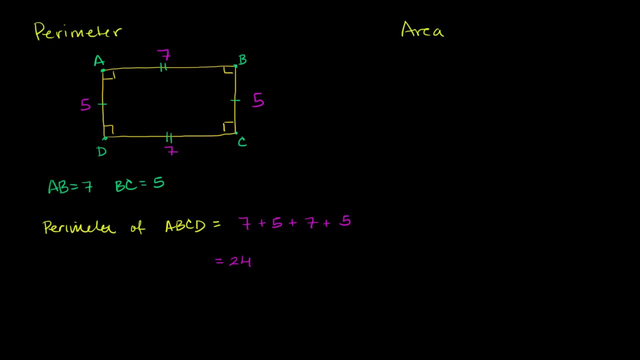 is a special case of a rectangle. A square has four sides and four right angles, and all of the sides are equal. So let me draw a square here, My best attempt. So this is A, B, C, D And we're going. 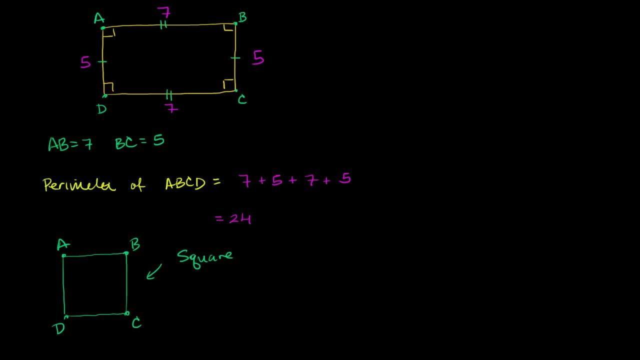 to tell ourselves that this right here is a square, And let's say that this square has a perimeter, So a square has a perimeter of 36.. So, given that, what is the length of each of the sides? Well, all the sides are going to have the same length. 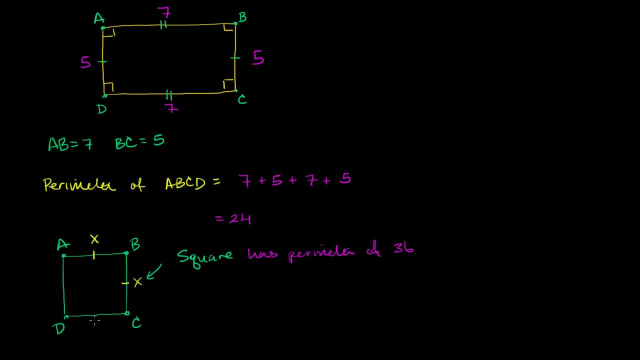 Let's call them x. So if AB is x, then BC is x, then DC is x and AD is x, All of the sides are congruent. All of these segments are congruent. They all have the same measure. We call that x. 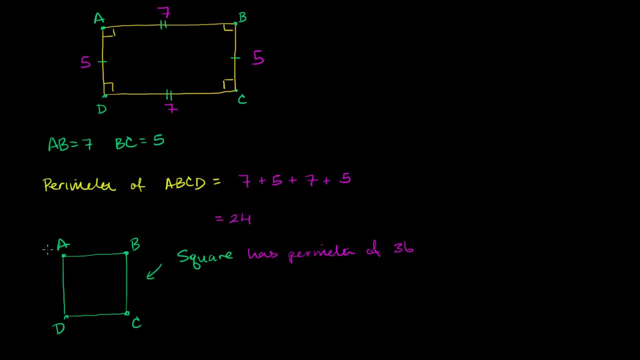 Given that, what is the length of each of the sides? Well, all the sides are going to have the same length. Let's call them x. So if ab is x, then bc is x, then dc is x and ad is x. 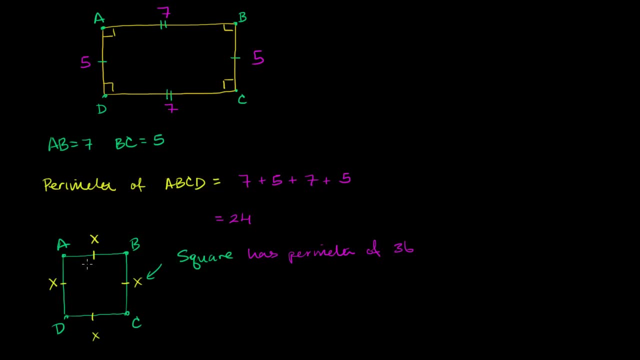 All of the sides are congruent, All of these segments are congruent. They all have the same measure. We call that x. So if we want to figure out the perimeter here, it'll just be x plus x plus x plus x or 4x. 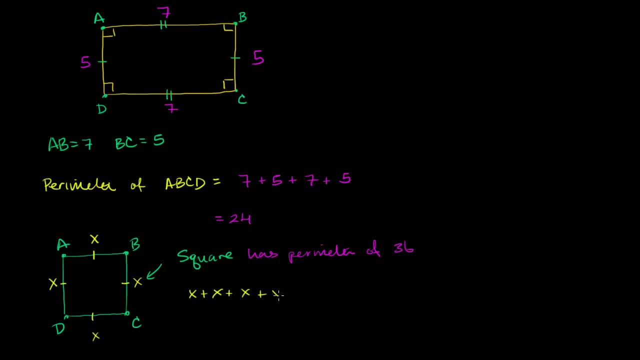 Let me write that x plus x plus x plus x, which is equal to 4x, which is going to be equal to 36.. They gave us that in the problem And to solve this, 4 times something is 36.. 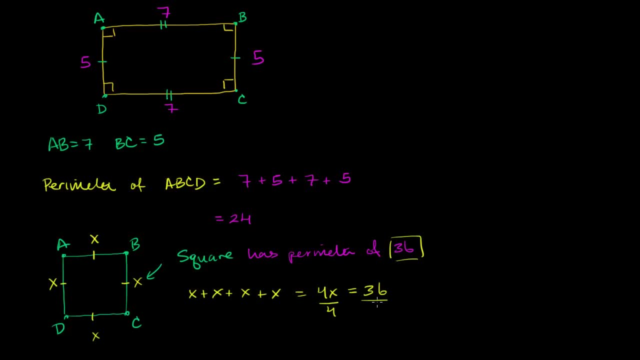 You could solve that probably in your head, But we could divide both sides by 4.. And you get: x is equal to 9.. So this is a 9 by 9 square. This width is 9,, this is 9, and then the height right over here. 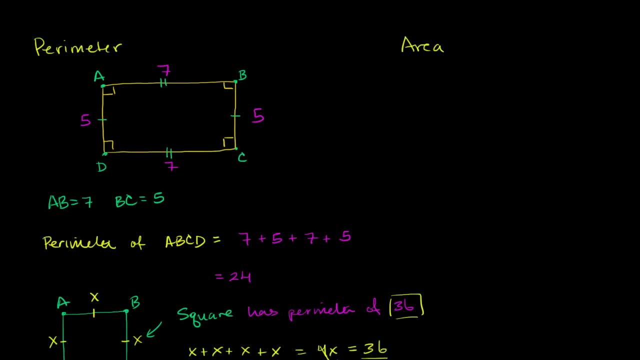 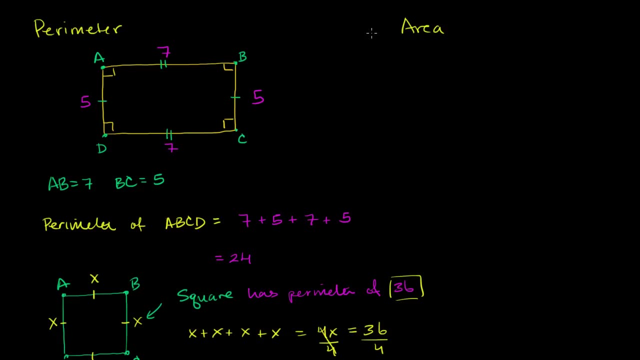 is also 9.. So that is perimeter. Area is kind of a measure of how much space does this thing take up in two dimensions? And one way to think about area is if I have a 1 by 1 square. So this is a 1 by 1 square. 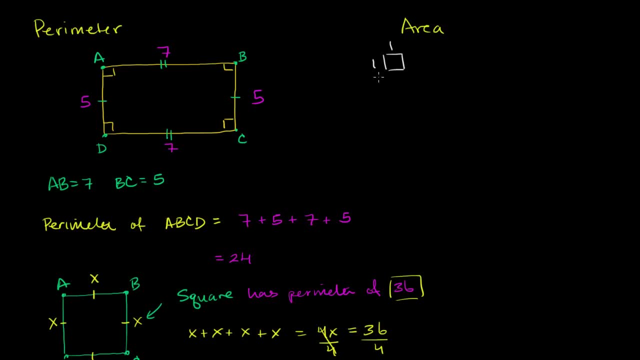 And when I say 1 by 1, it means you only have to specify two dimensions for a square or a rectangle, because the other two are going to be the same. So, for example, you could call this a 5 by 7 rectangle. 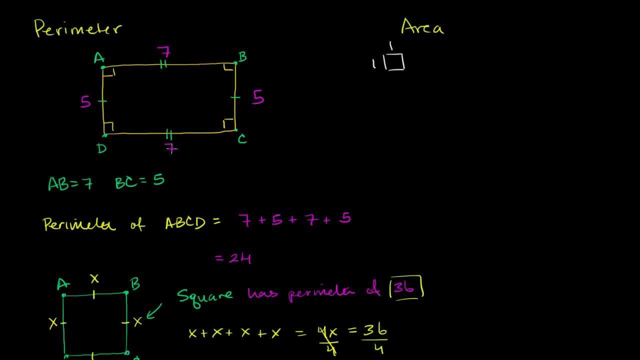 because that immediately tells you: OK, this side is 5 and that side is 5.. This side is 7 and that side is 7.. And for a square you could say it's a 1 by 1 square, because that specifies all of the sides. 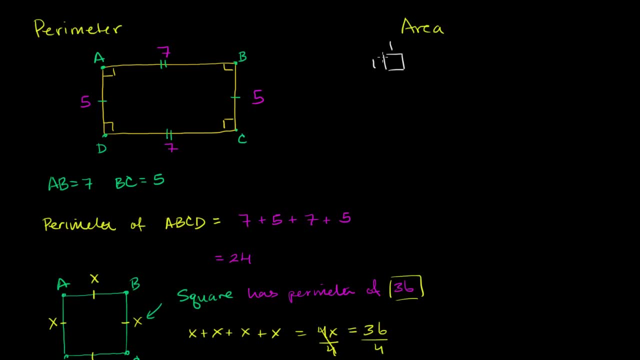 You could really say for a square, a square where one side is 1, then really all of the sides are going to be 1.. So this is a 1 by 1 square, And so you can view the area of any figure. 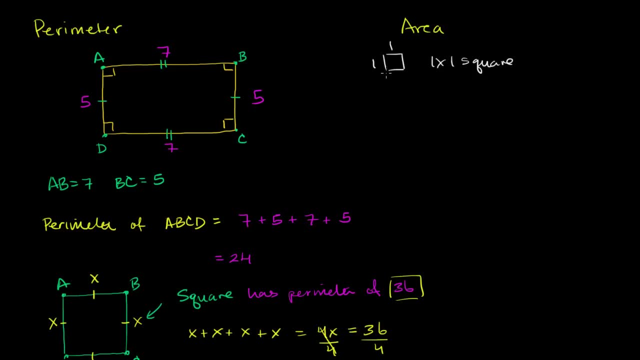 as how many 1 by 1 squares can you fit on that figure? So, for example, if we were going back to this rectangle right here and I wanted to find out the area of this rectangle and the notation we can use for area, 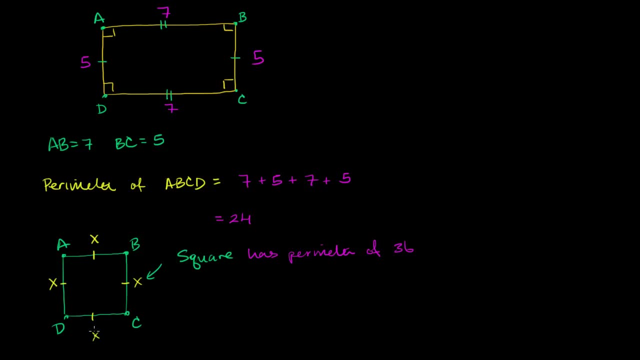 So if we want to figure out the perimeter here, it'll just be x plus x plus x plus x or 4x. Let me write that x plus x plus x plus x, which is equal to 4x, Which is going to be equal to 36.. 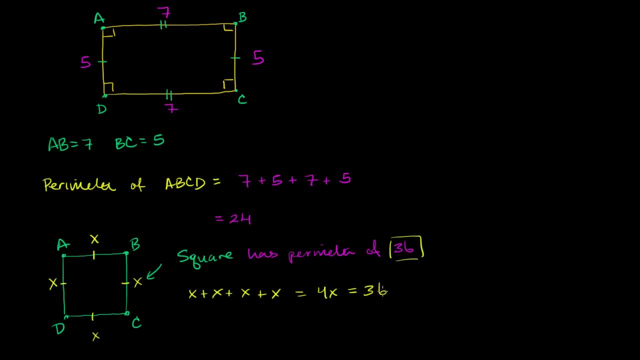 They gave us that in the problem. And to solve this 4 times, something is 36.. You could solve that probably in your head, But we could divide both sides by 4. And you get x is equal to 9.. So this is a 9 by 9 square. 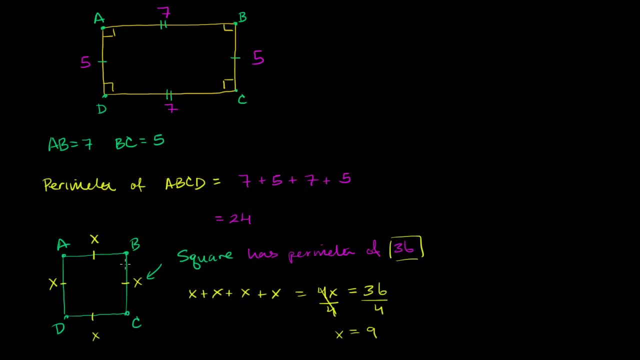 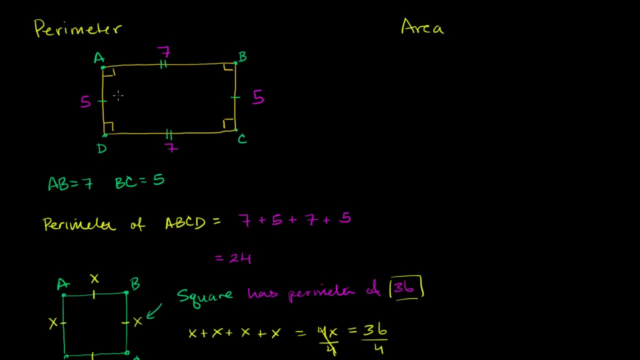 This width is 9.. This is 9.. And then the height right over here is also 9.. So that is perimeter. Area is kind of a measure of how much space does this thing take up in two dimensions? And one way to think about area is if I have a 1 by 1 square. 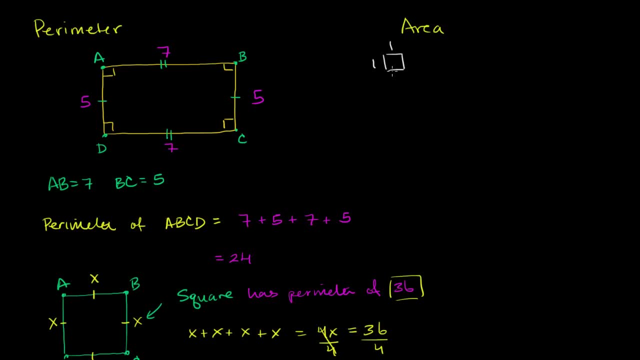 So this is a 1 by 1 square, And when I say 1 by 1, it means you only have to specify two dimensions for a square or a rectangle, because the other two are going to be the same. So, for example, you could call this a 5 by 7 rectangle. 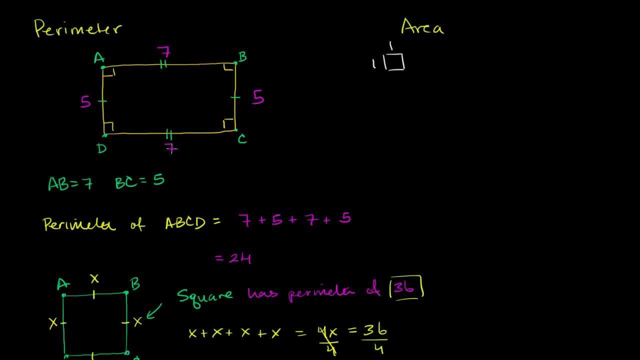 because that immediately tells you: OK, this side is 5 and that side is 5.. This side is 7 and that side is 7.. And for a square you could say it's a 1 by 1 square, because that specifies all of the sides. 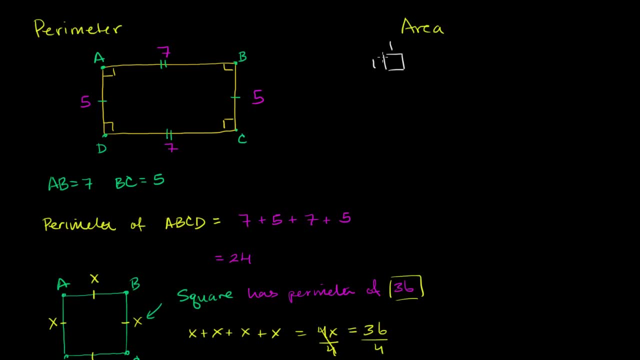 You could really say for a square, a square where one side is 1, then really all of the sides are going to be 1.. So this is a 1 by 1 square, And so you can view the area of any figure. 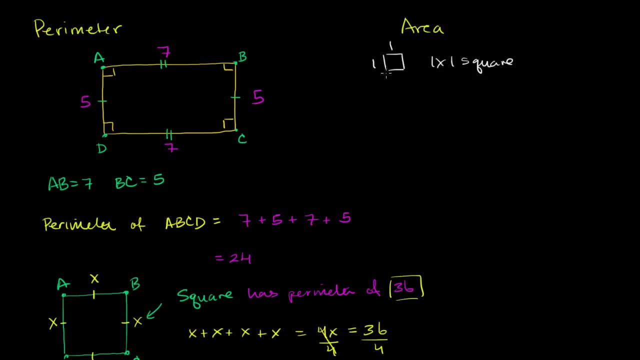 as how many 1 by 1 squares can you fit on that figure? So, for example, if we were going back to this rectangle right here and I wanted to find out the area of this rectangle and the notation we can use for area, 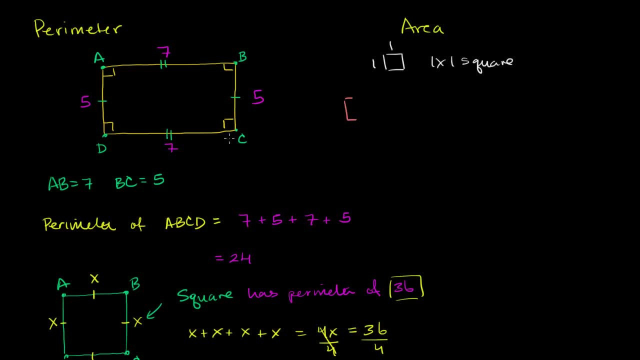 is put something in brackets. So the area of rectangle A, B, C D, A, B, C D is equal to the number of 1 by 1 squares we can fit on this rectangle. So let's try to do that just manually. 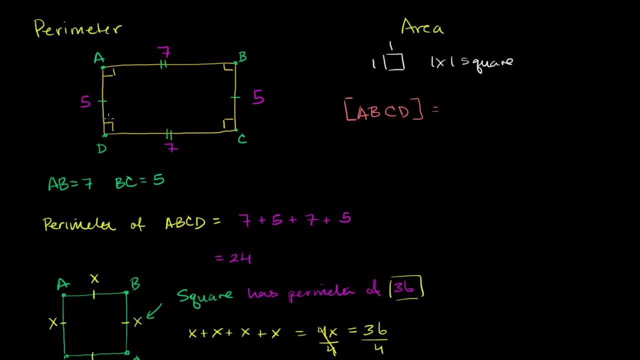 I think you already might get a sense of how to do it a little bit quicker. But let's put a bunch of 1 by 1.. So let's see, We have 5 1 by 1 squares this way and 7 this way. 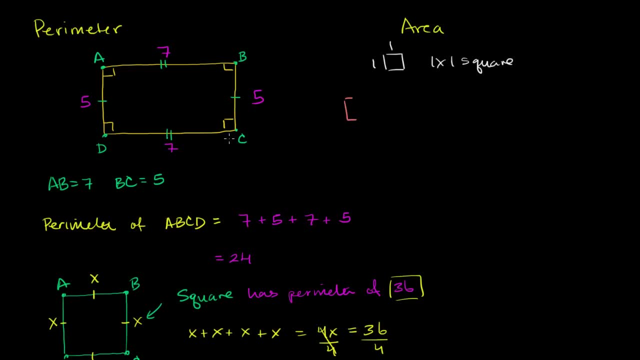 is put something in brackets. So the area of rectangle A, B, C, D is equal to the number of 1 by 1 squares we can fit on this rectangle. So let's try to do that just manually. I think you already might get a sense of how. 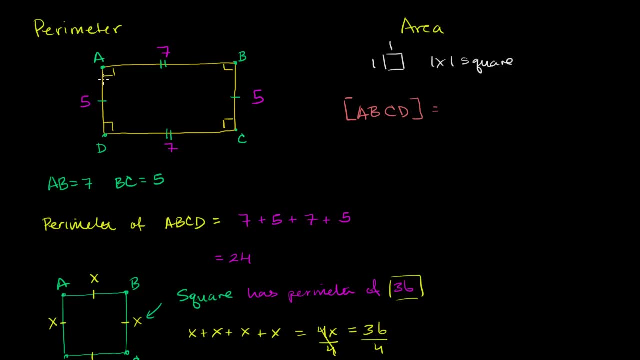 to do it a little bit quicker, But let's put a bunch of 1 by 1.. So let's see We have 5 1 by 1 squares this way and 7 this way. So I'm going to try my best to draw it neatly. 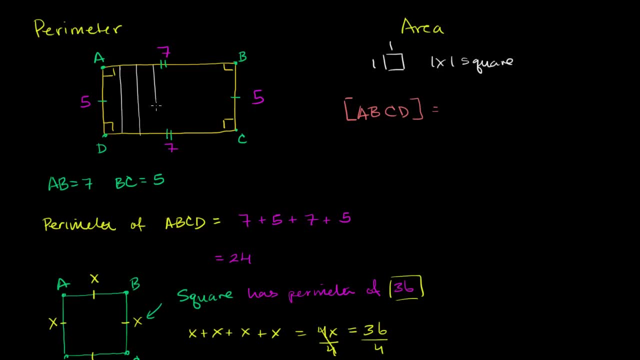 So that's 1,, 2,, 3,, 4,, 5,, 6,, 7.. 6 and then 7.. 1,, 2,, 3,, 4,, 5,, 6,, 7.. 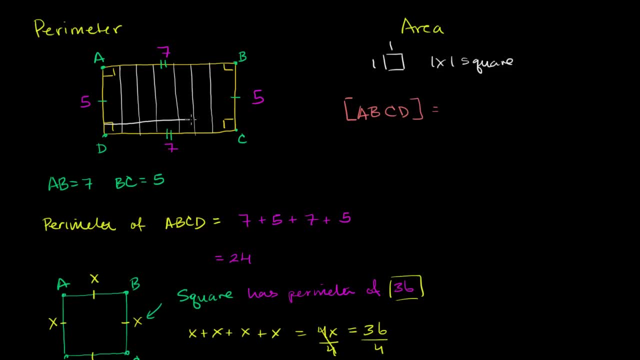 So going along one of the sides, if we just go along one of the sides like this, you could put 7 just along one side, just like that. And then over here, how many can we see? We see that's 1 row, that's 2 rows. 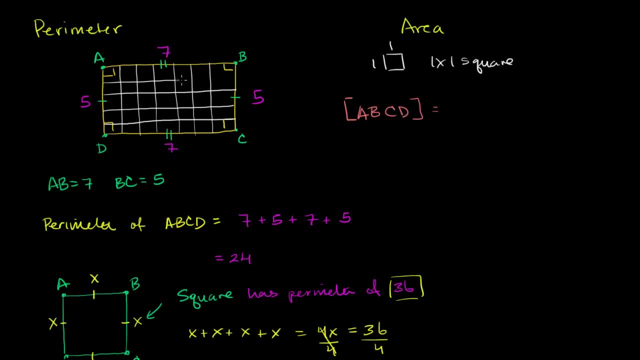 then we have 3 rows and then 4 rows, and then 5 rows: 1,, 2,, 3,, 4, 5.. And that makes sense, because this is 1,, 1,, 1,, 1, 1.. 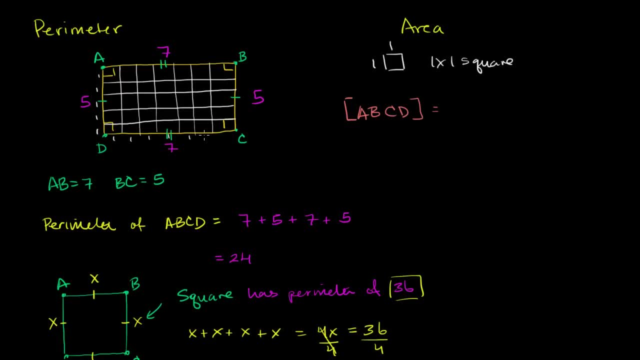 It should add up to 5.. These are 1, 1, 1, 1, 1, 1, 1.. It should add up to 7.. Yep, there's 7.. So this is 5 by 7.. 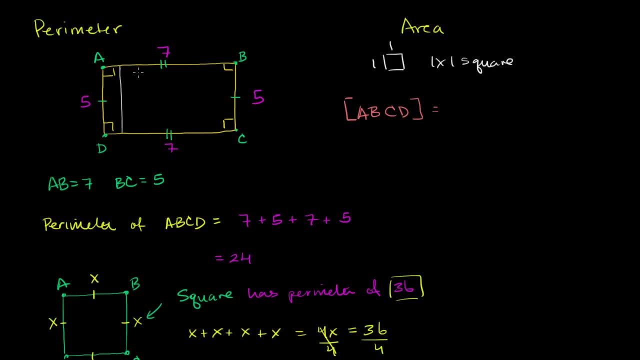 So I'm going to try my best to draw it neatly. So that's 1,, 2,, 3,, 4,, 5, 6. 7.. 1,, 2,, 3,, 4,, 5,, 6,, 7.. 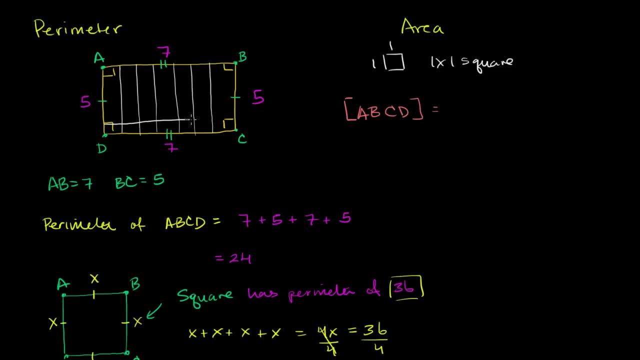 So, going along one of the sides, if we just go along one of the sides like this, you could put 7 just along one side, just like that. And then over here, how many can we see? We see that's 1 row, that's 2 rows, 2 rows. 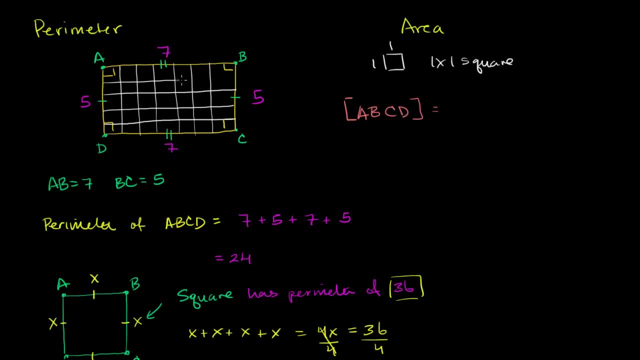 Then we have 3 rows and then 4 rows, and then 5 rows: 1,, 2,, 3,, 4, 5.. And that makes sense, because this is 1,, 1,, 1,, 1, 1.. 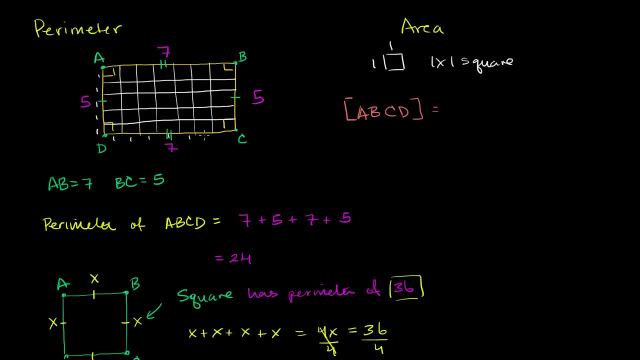 Should add up to 5.. These are 1, 1, 1, 1, 1, 1, 1.. Should add up to 7.. Yep, there's 7.. So this is 5 by 7.. 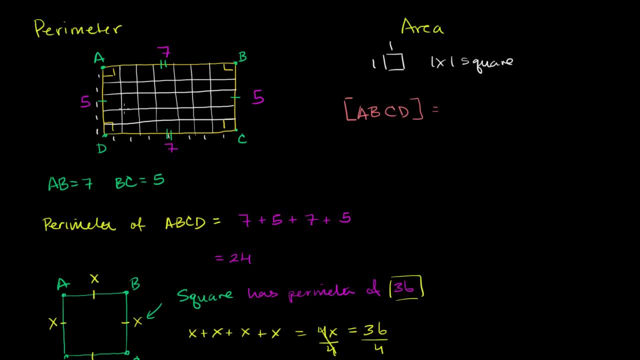 And then you could actually count these. And this is kind of straightforward multiplication. If you wanted to know the total number of cubes here, you could count it. Or you'd say: well, look, I have 5 rows, 7 columns. 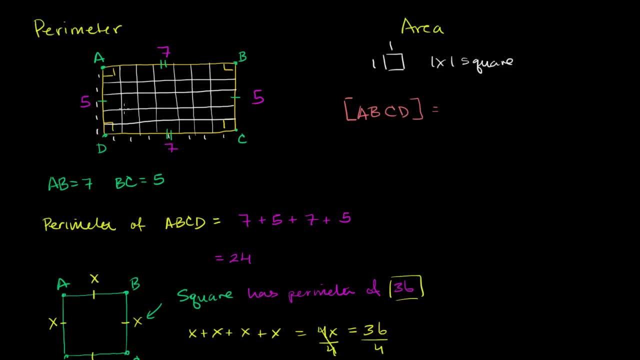 And then you could actually count these. And this is kind of straightforward multiplication. If you wanted to know the total number of cubes here, you could count it. Or you could say: well, look, I have 5 rows, 7 columns. 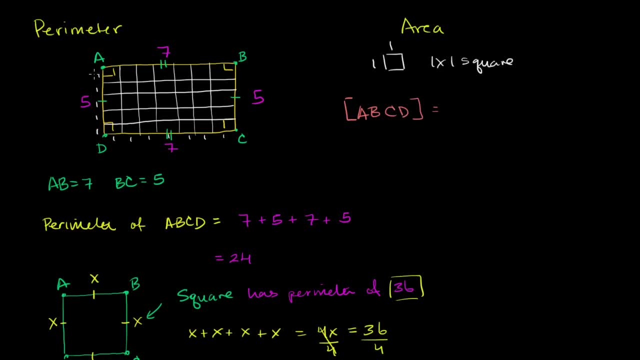 I'm going to have 35, did I say cubes squares? I have 5 squares in this direction, 7 in this direction, so I'm going to have 35 total squares. So the area of this figure right over here is 35.. 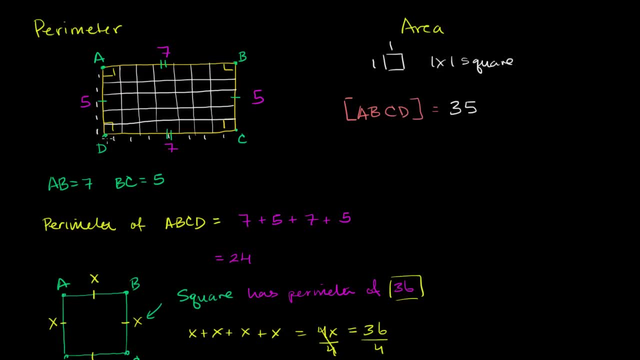 And so the general method. you could just say: well, I'm just going to take one of the dimensions and multiply it by the other dimension. So if I have a rectangle, let's say the rectangle is 1, half by 2.. 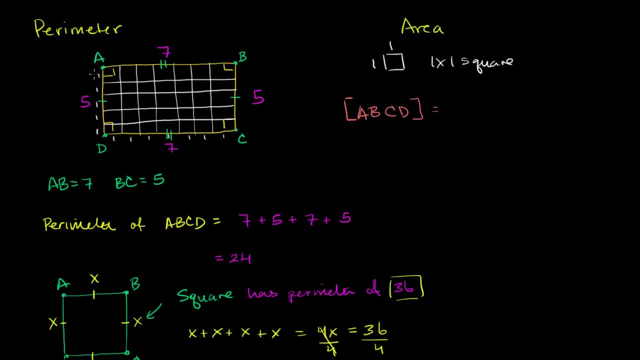 I'm going to have 35.. Now did I say cube squares? I have 5 squares in this direction, 7 in this direction. So I'm going to have 35 total squares. So the area of this figure right over here. 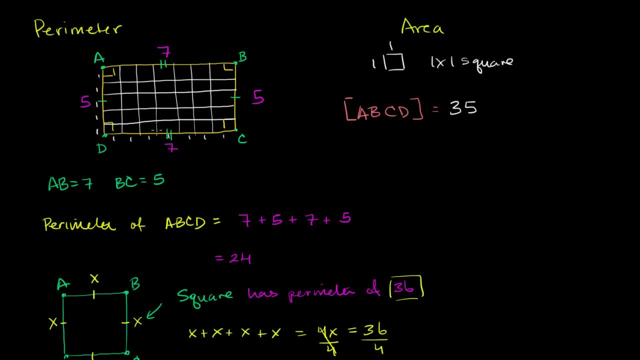 is 35.. And so the general method. you could just say: well, I'm just going to take one of the dimensions and multiply it by the other dimension. So if I have a rectangle, let's say the rectangle is 1, half by 2.. 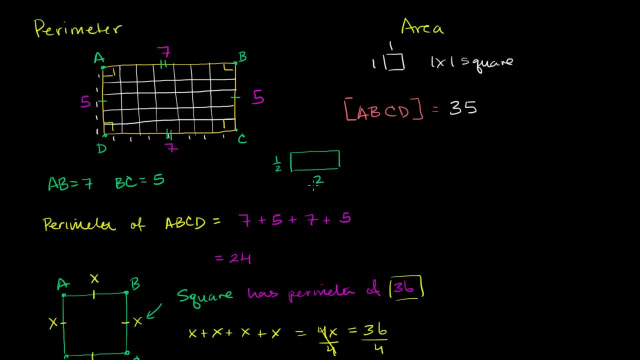 Those are its dimensions. Well, you could just multiply it. You'd say 1 half times 2, the area here is going to be 1.. And you might say: well, what does 1 half mean? Well, it means in this dimension, I can only fit half. 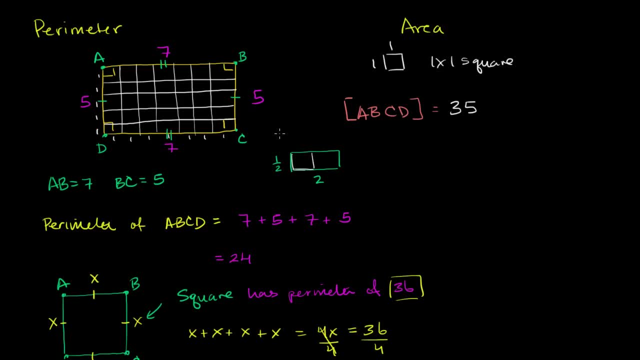 I can only fit half. I can only fit half of a 1 by 1 square. So if I want to do the whole 1 by 1 square, it's a little distorted here. It would look like that, So I'm only doing half of 1.. 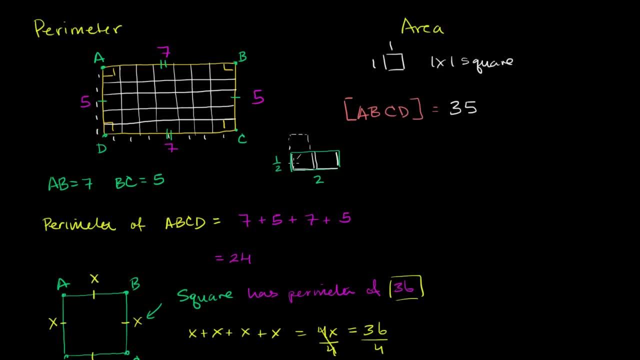 I'm doing another half of 1 just like that, And so when you add this guy and this guy together, you are going to get a whole 1.. Now, what about area of a square? Well, a square is just a special case. 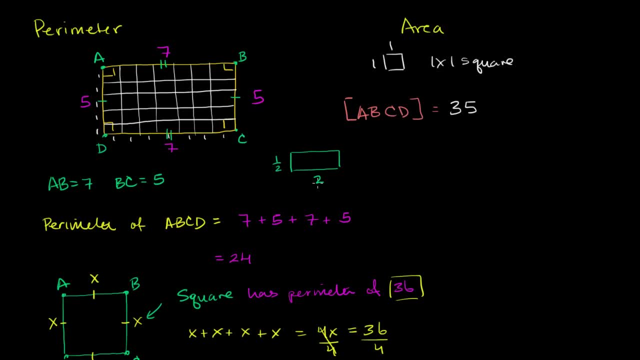 Those are its dimensions. Well, you could just multiply it. You say 1 half times 2, the area here is going to be 1.. And you might say: well, what does 1 half mean? Well, it means in this dimension. 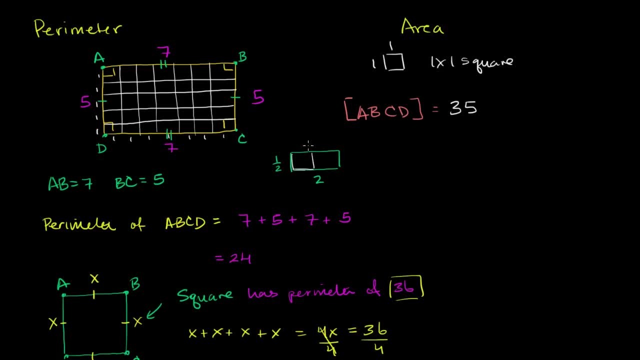 I can only fit 1 half of a 1 by 1 square. So if I want to do the whole 1 by 1 square, it's a little distorted here. it would look like that, So I'm only doing 1 half of 1.. 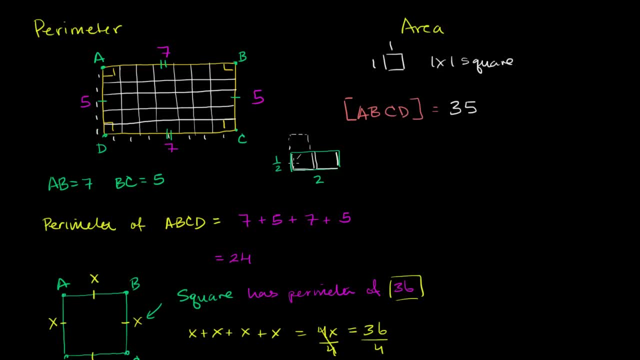 I'm doing another 1, half of 1, just like that, And so when you add this guy and this guy together, you are going to get a whole 1.. Now, what about area of a square? Well, a square is just a special case. 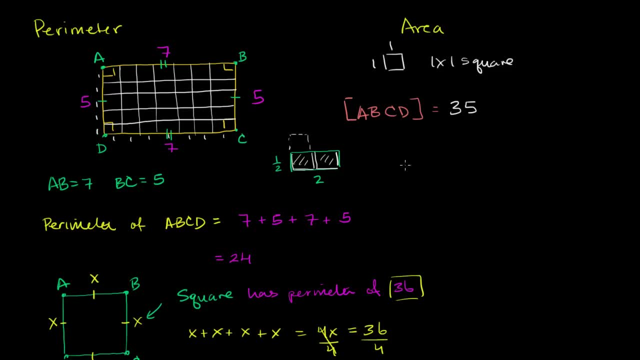 where the length and the width are the same. So if I have a square, let me draw a square here And let's call that x, y, z, I don't know. Let's make this s And let's say I wanted to find the area. 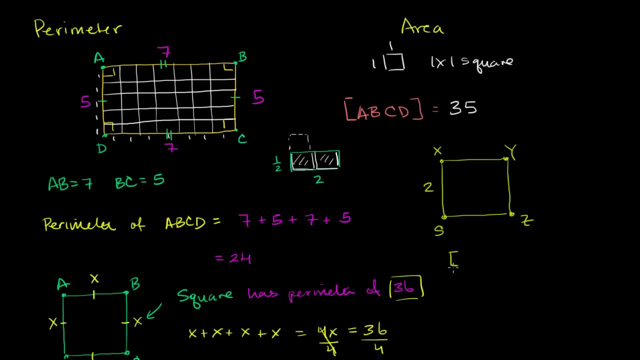 And let's say, I know one side over here is 2.. So xs is equal to 2. And I want to find the area of x, y, zs. So once again, I use the brackets to specify the area of this figure, of this polygon. 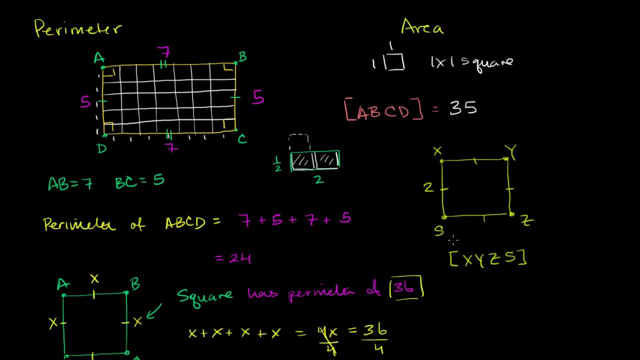 right here, this square, And we know it's a square, We know all the sides are equal. Well, it's a special case of a rectangle where we would multiply the length times the width. We know that they're the same thing. 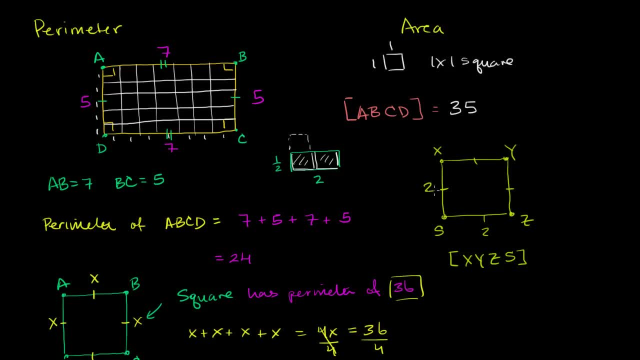 If this is 2,, then this is going to be 2.. So you just multiply 2 times 2.. Or, if you want to think of it, you square it, which is where the word comes from squaring something. So you multiply 2 times 2,, which is equal to 2 squared. 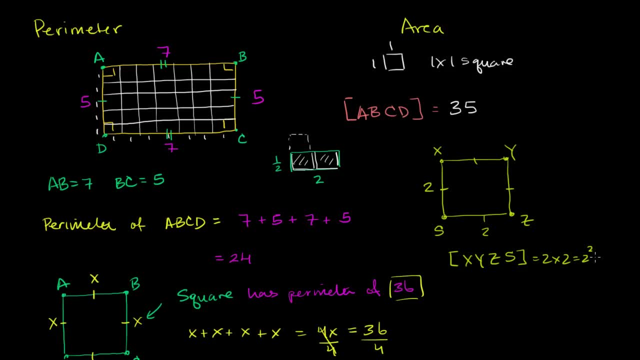 That's where the word comes from: finding the area of a square which is equal to 4.. And you can see that you can easily fit four 1 by 1 squares on this 2 by 2 square And I've got one square point here. I've got zero square point here And I'm just going to divide this by 1, and I'm just going to go and take it to that square which is square 2,, square 2, square 1,, square 1, square 3.. And we do that. And my idea is that when we do this particular product in our set and we do the same thing in our set and we change the data set to square 2, square 1, square 2, square 1, square 2, square 1, square 1, square 2, square 3.. Now I'm going to go and try to find the area of x, y, z and oh, I have it.